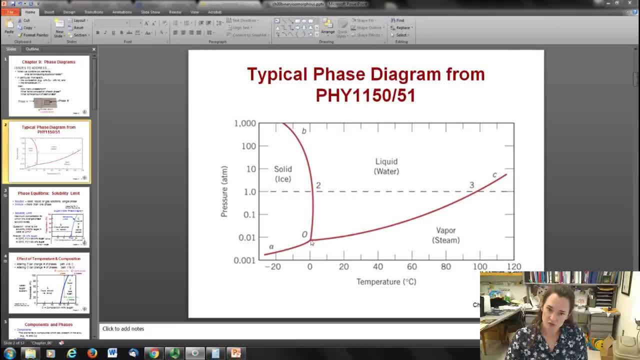 to the gas, And then you have here the triple point. Now remember that on the line, while you're sitting on the line, that the material can exist in both phases at once, And so what happens is when water goes from a solid to a liquid, it takes energy to kind of heat. 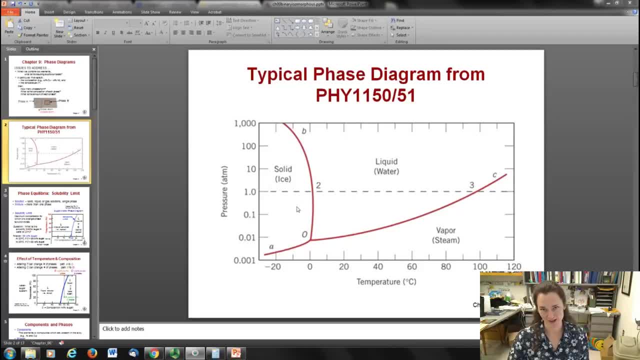 it up And that Q is equal to MC delta T. And then, once it reaches zero degrees C, it won't change temperature anymore until it's completely melted. Okay, So it holds steady at that temperature. And while it's holding steady at that temperature, it'll be in the process of melting and you'll have both solid. 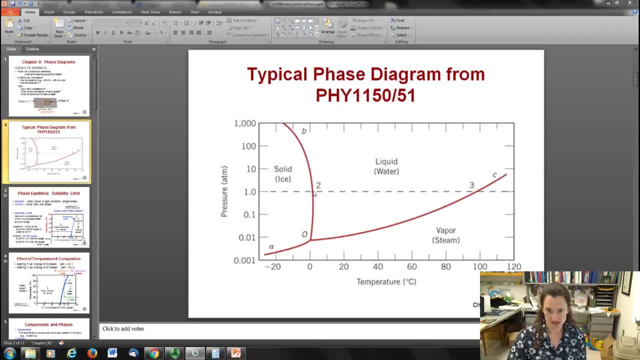 and liquid while it holds at that temperature. So that's kind of as represented here on the line. It's where the material can coexist in the two phases, Where all these lines intersect. that's known as the triple point. And the really fun thing- 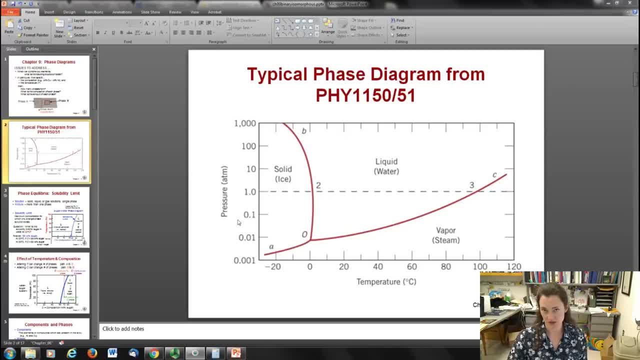 about the triple point of water is, of course it can be in all three phases at once- solid, liquid and gas- all at the same time, which is kind of fun. So that's a little bit of a reminder of what's going on with material in these kinds of phase. 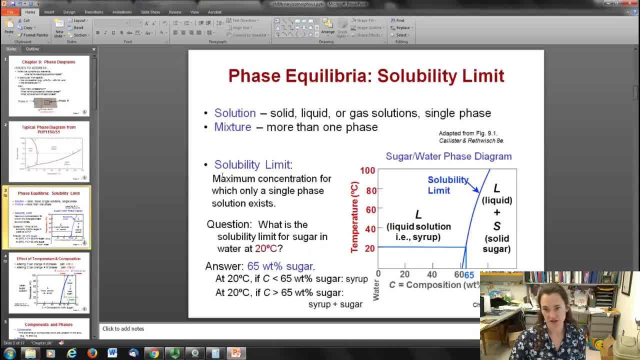 diagrams. Now there's another phase diagram that you might have looked at in some elementary chemistry classes or in high school or whatever, And that has to do with the percent composition of the material versus the temperature. So instead of plotting pressure versus temperature for 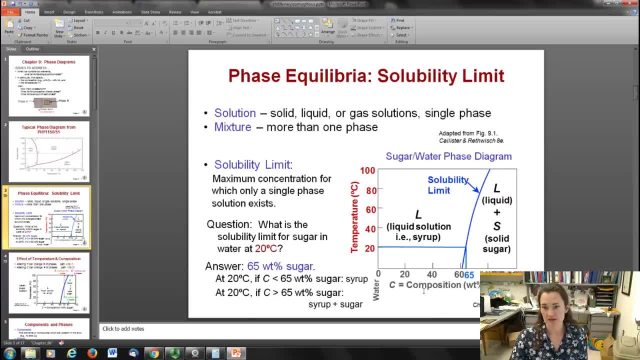 example, as we saw in the water phase diagram, then you can change the composition versus temperature. So this phase diagram shown here is the sugar water phase diagram And so as you go along the bottom of this plot, you're increasing the weight percentage of sugar in your sugar water solution. 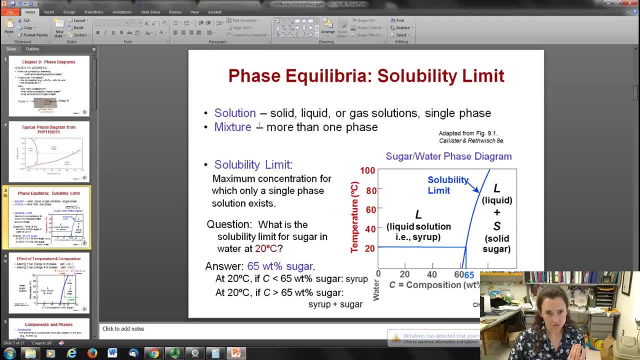 Okay, So from this you're getting a mixture, So there could be more than one phase going on. For example, here's your solubility limit. That's the solubility limit line, that kind of arcing line on the last right-hand third of the graph. 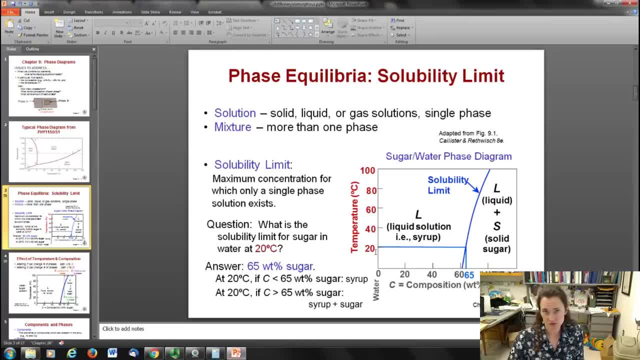 And what happens is that at a given temperature- let's pick room temperature, for example- as you add sugar, you can get the sugar to dissolve into the liquid phase up to a certain point, up to a certain weight percentage, And then, past that, you're not going to be able to get the sugar to dissolve anymore. 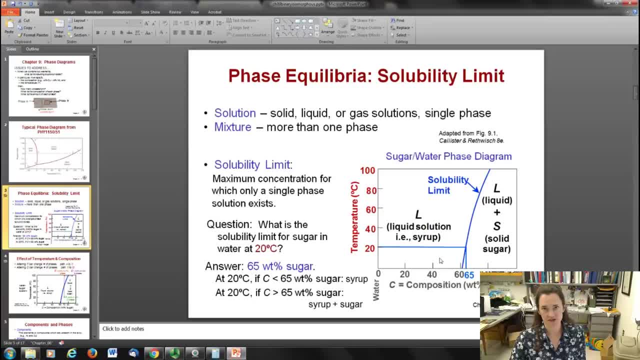 It's going to stay in its solid state, just as a precipitate, for example, on the bottom of your glass or bowl or whatever. So the limit, the weight percentage limit, for that is indicated by the line And if you go across to the intersection at twenty degrees Celsius, you can see. 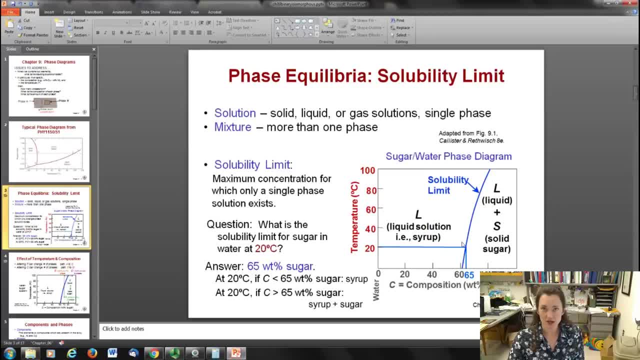 that that intersection happens at about sixty-five weight percent for the sugar water solution. So what can happen is, let's say, that you heat your solution up to a certain weight percentage and you're going to want to add a little bit of water to the solution. 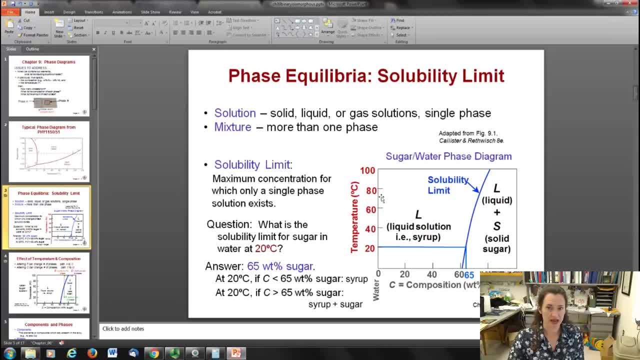 So what can happen is, let's say that you heat your solution up to a certain weight percentage and you're going to want to add a little bit of water to the solution. So what can happen is, let's say that you heat your solution up to a certain weight percentage and you're going to want to add a little bit of water to the solution. 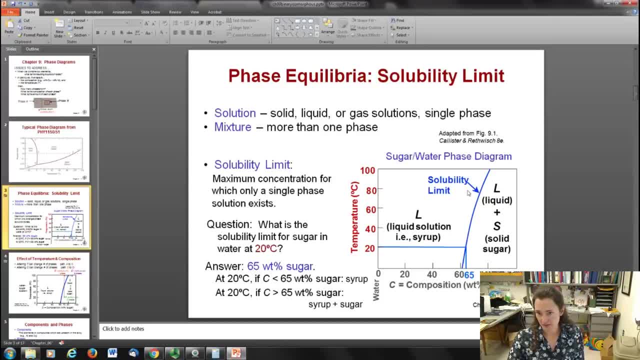 So what can happen is, let's say, that you heat your solution up to, say, eighty or ninety degrees C. Okay, well now if you're at eighty degrees C, you can see that your limit is the higher weight percentage. Okay, so you can mix more sugar in. 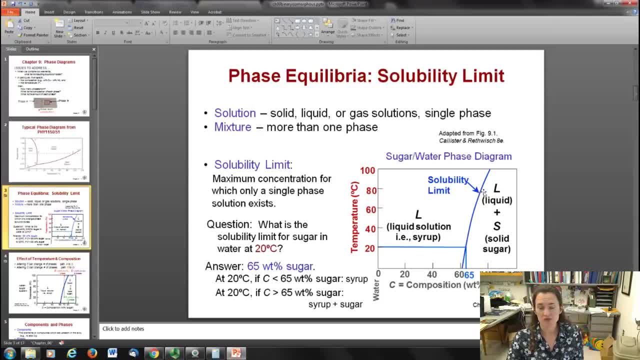 So let's say that you go up to eighty degrees C and you mix more sugar in, but then you cool it off, And as you cool it off, some of that sugar that you got to successfully dissolve at eighty degrees C is going to precipitate out into little crystals on the bottom of your glass. 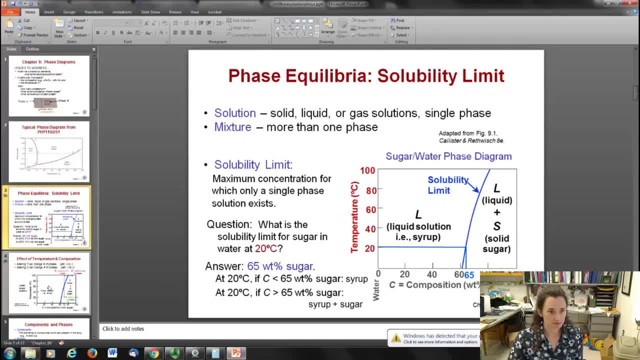 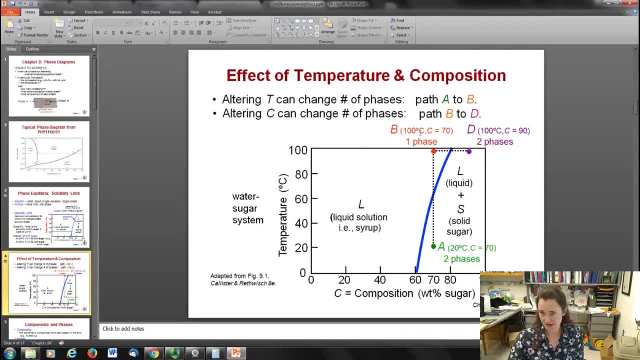 So that's kind of what's going on with that kind of phase diagram. So basically you're in a situation where, if you alter your temperature, you can change the number of phases. So, for example, if you go from A to B, here you're starting at a temperature of, say, 20 degrees. 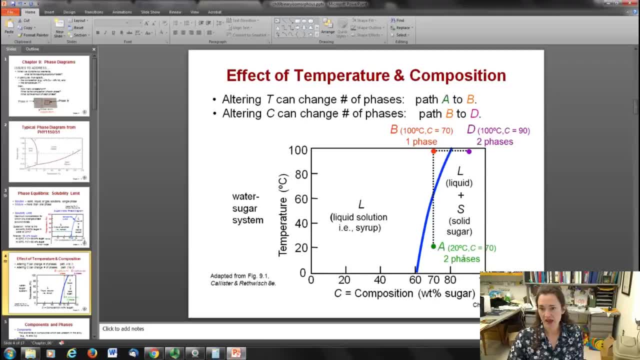 Celsius with 78% of sugar, and you've got two phases. You've got your liquid and your solid precipitates, And then if you go up, then you cross that line. you've heated it up and then some of that sugar that precipitated out of the solution will dissolve in to the liquid state, So that 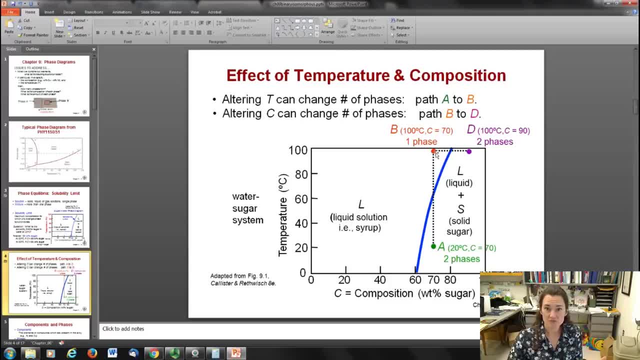 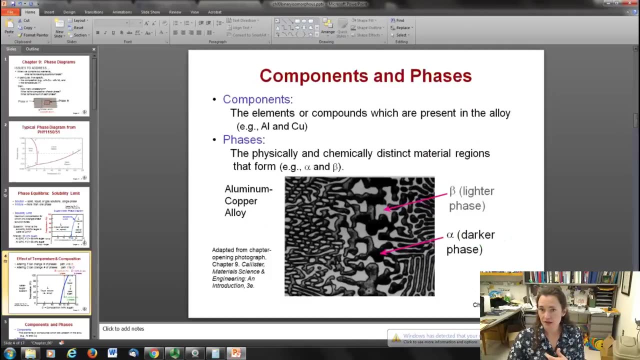 changes the number of phases from two to one. Now if you add more sugar and you go from B to D, then you're going to go from a liquid state to a liquid and a solid state where that sugar just won't dissolve in anymore. So that's kind of what's going on there. Now I wish I could say: 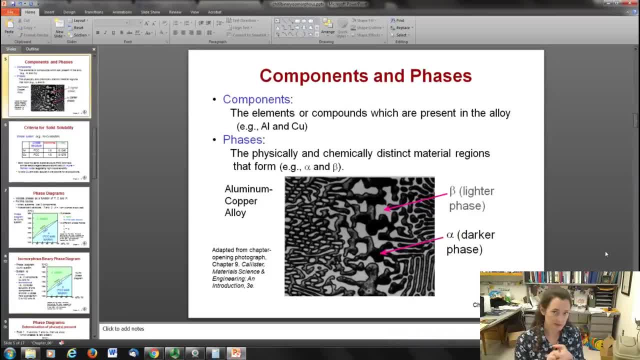 that all of the phase diagrams in material science were as happy smiley as that. But what happens in material science is that you get more than one kind of solid phase and they can actually have different structures. So, for example, this is an image of aluminum and 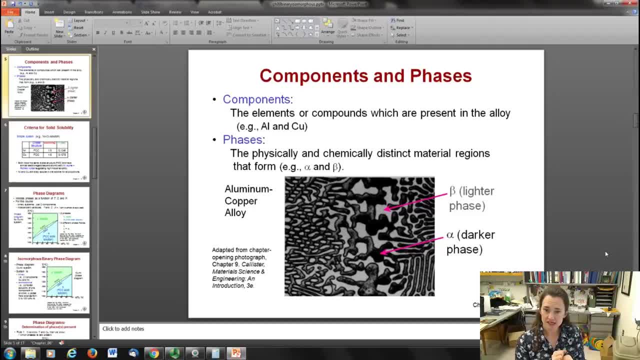 copper formed in an alloy, And you can see here that it's kind of a cool looking picture actually that there's two different phases present. One of the phases shows up as darker than the other, So the alpha phase actually has a dark color to it and the beta phase is a lighter color. And this is, I believe, from an SEM image. 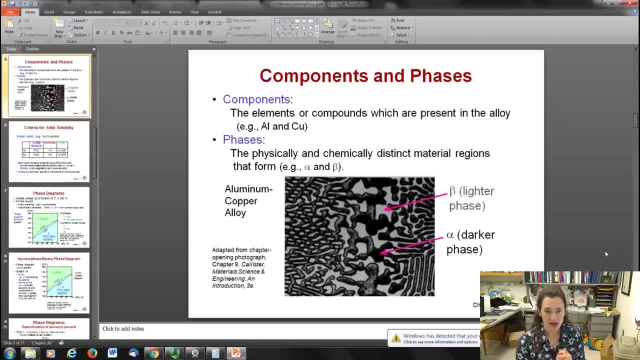 a scanning electron microscope image of the two phases. Okay, so those two phases they're both solids but they're physically and chemically distinct regions that form. okay. So they might have different crystalline structures and they also are different chemically. They have different. 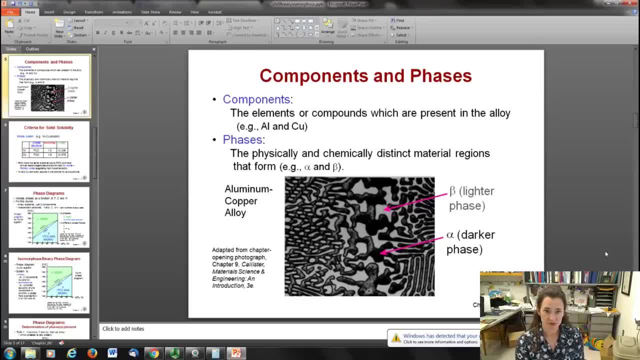 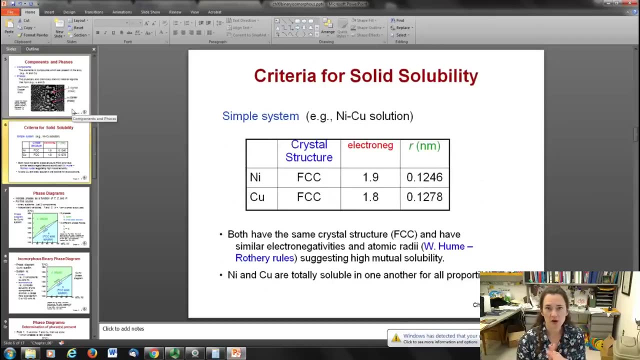 chemical compositions. Perhaps one of them, for example, probably the copper. the alpha phase is copper-rich, and then the beta phase has more aluminum. okay, So it's a lighter density phase as well. All right, but before we embark on the really super fun phase diagrams that you can get into, 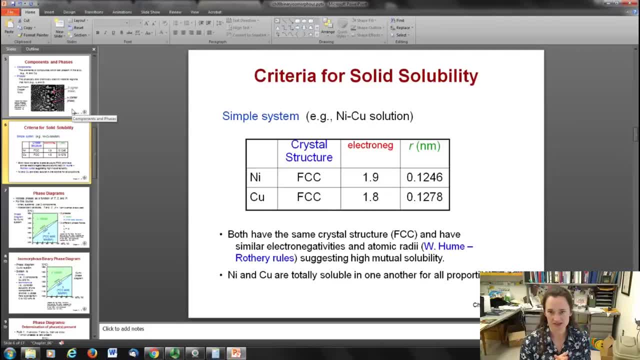 in material science. let's start off with the simplest system possible, so you can get used to looking at them and so you can learn how to do some of the techniques for analysis. So the simplest thing that you can do in material science is to have a system with two components. 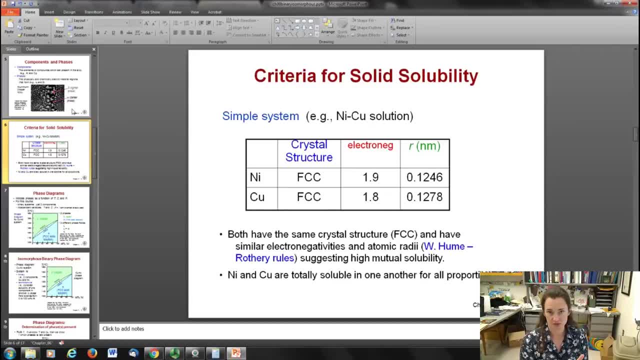 like nickel and copper that are completely soluble in one another. all right, Now. they both have the same crystalline structure, they're both FCC and they have similar electronegativities and atomic radii. So you might remember the Hume-Rothory rules that we covered in a previous. 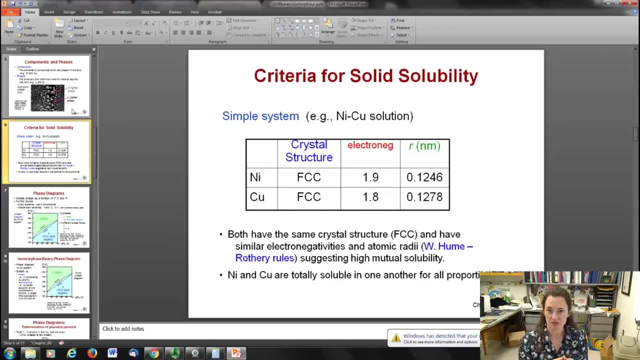 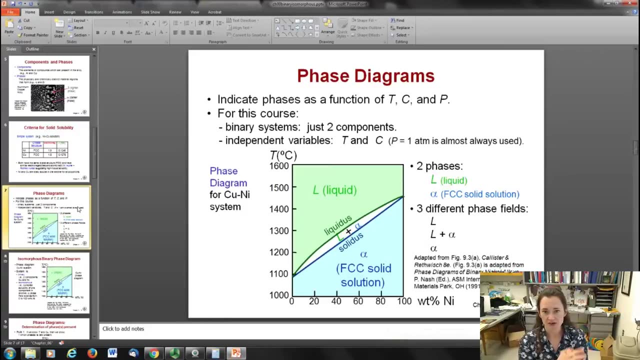 lecture. So these two things have very high mutual solubility, all right, So they're totally soluble for all proportions, which is awesome and, as we'll see, really unusual actually. So if you look at the copper-nickel phase diagram, what you can do is you can indicate the phases as 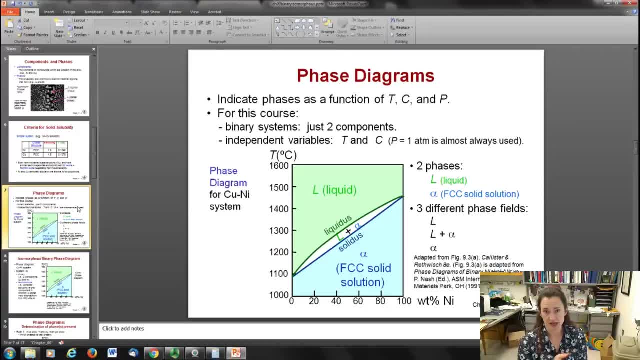 a function of temperature, composition and pressure. You can. You can plot the pressure too, like we did for the water phase diagram, But for this course those can get kind of complicated and complex. So for this course we're just going to look at the copper-nickel phase diagram. 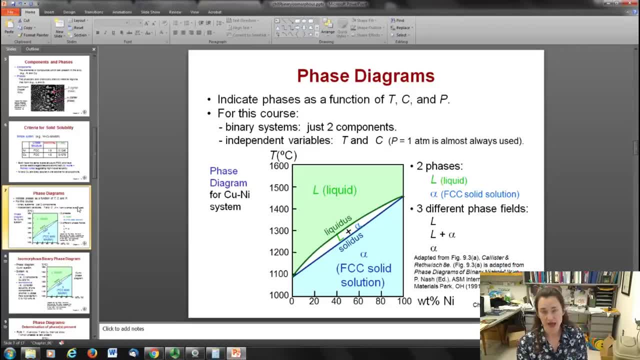 and we're going to look at binary systems with two components like copper-nickel, and we're going to only examine the independent variables of temperature and percent composition And we're just going to hold the pressure at one atmosphere, which is what the standard kind of is for. 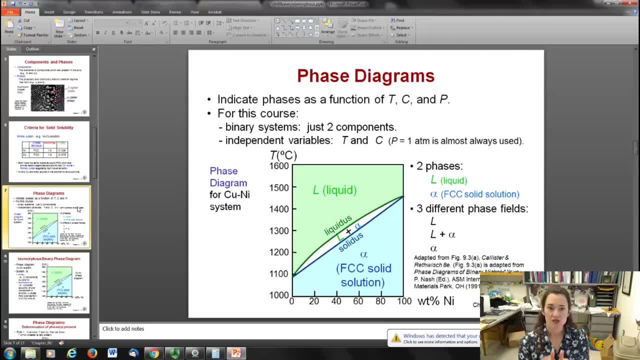 comparison anyway, since we're at one atmosphere here. okay, So if we do that for copper-nickel, then this is what the phase diagram looks like. You can see the liquid portion is in green and the solid portion is in blue, And we're going to call the 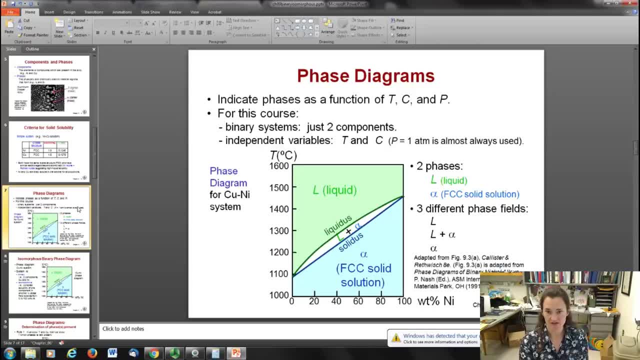 solid phase here, the alpha phase. okay, So this is the alpha solid phase And it's an FCC solid solution. Along the bottom of the graph is plotted the percent change in weight, percent of nickel. So you start all the way here on the left-hand side where you've got all copper, and then, as 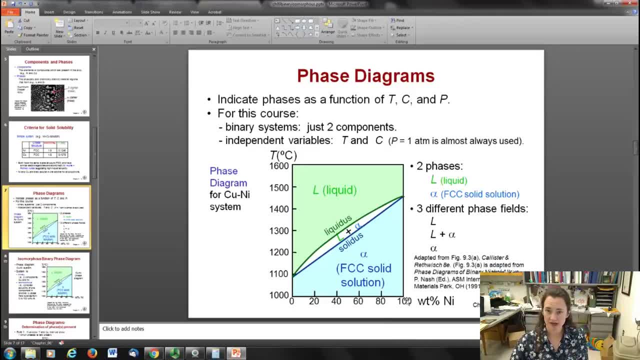 you increase your weight percentage, you end up eventually on the right-hand side where you have pure nickel. okay, Now the temperature increases. here We just zoomed in on the high temperature near the melting point And we're going to look at the copper-nickel phase here And we're going to 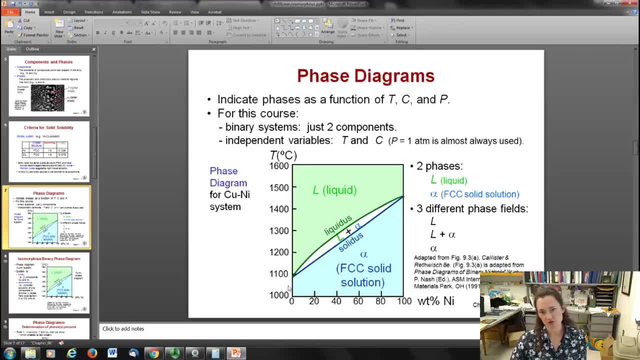 see that it's a solid point for these percentages because of course, below that, below a thousand degrees C, of course it's a solid, And above where it goes, where nickel melts, of course it's a liquid. okay, So there you go. Now you can see, if you look at this phase diagram, that copper. 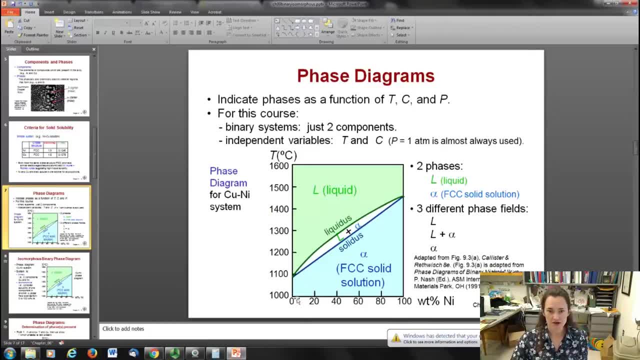 and nickel have different melting points. okay, If you're over here on the left-hand side at zero weight percent nickel, then that's the melting point of copper. okay, And if you're over here on nickel, then you read it off: that's the melting point of nickel. okay, But you can see that in. 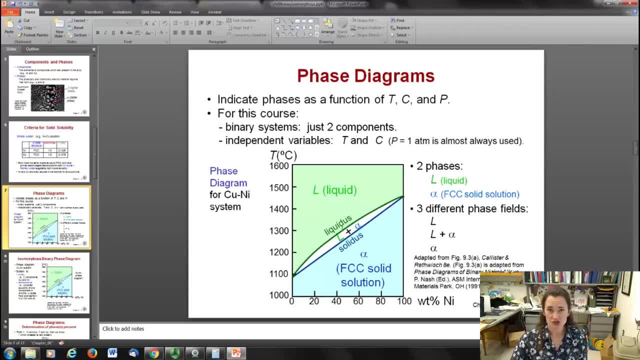 the intermediate region here, because the copper and the nickel do have different melting points. then you're going to get a region in between your liquidus and your solidus lines where you have a mixed phase, where you have some liquid and some alpha phase material, And this is because copper 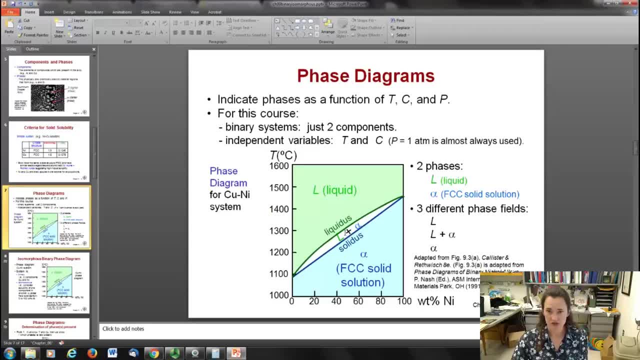 and nickel are different materials and they don't have the same melting point. So you're going to get this region where you've got a mix of liquid and solid, as one catches up to the other, if that makes sense. okay, So liquid phase, alpha phase, solid phase, liquid plus alpha phase, a mix of 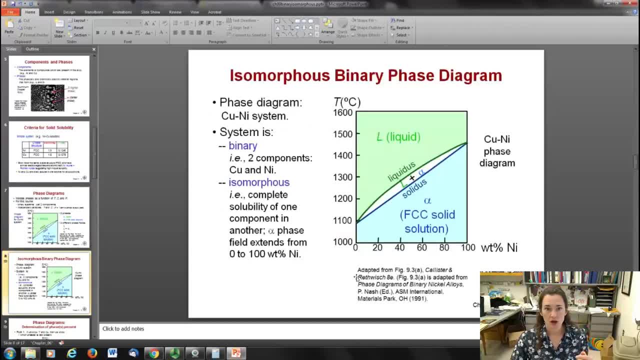 liquid plus solid. All right, this is called an isomorphous binary phase diagram. okay, It's binary because it's got two components: copper and nickel. It's isomorphous because you have complete solubility of one phase and one phase, So you're going to get a mix of liquid and solid. 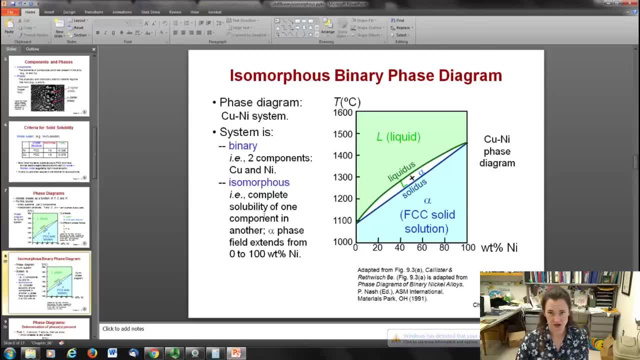 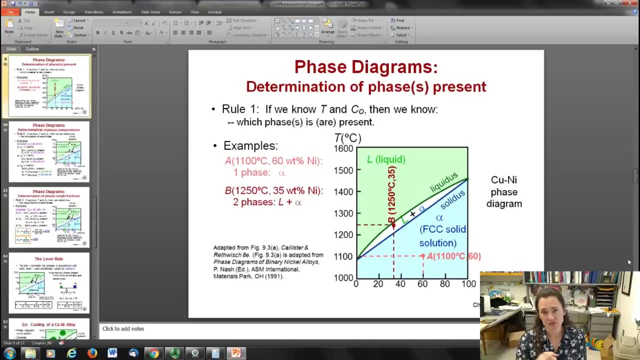 in one component and the other. okay, Complete is completely soluble means isomorphous, So this is an isomorphous binary phase diagram. Okay, so here's how to read these suckers. Rule number one: if you know the temperature and the percent composition, then you know which phases are. 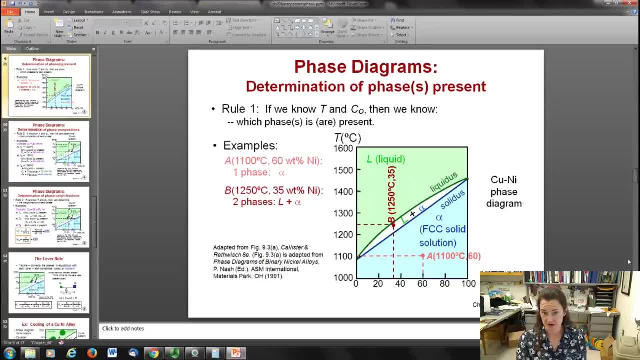 present. Okay. so, for example, if we go to point A here and we know that we've got 60 weight percent nickel at a temperature of 1100 degrees Celsius, then we know that we've got a mix of liquid and solid at 1200 degrees C. then I can figure out what phase I'm at, okay, And that phase is, of course. 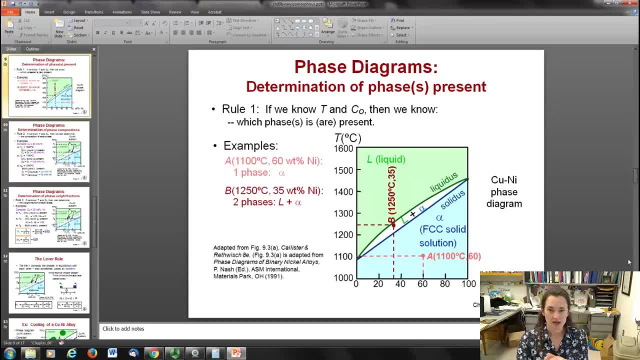 the FCC solid solution, the alpha phase. all right Now, if I have a 35 percent nickel solution at 1250 degrees C, then I can go and I can see what my phase is, And at that point I'm in the 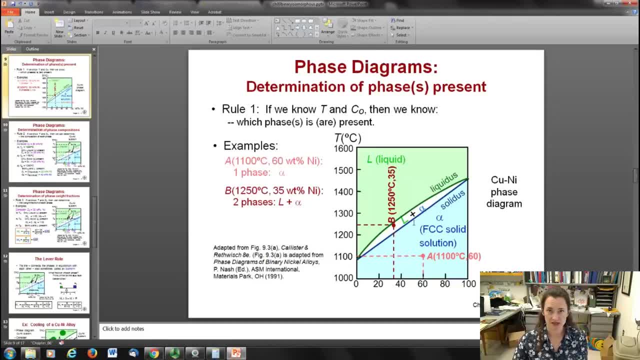 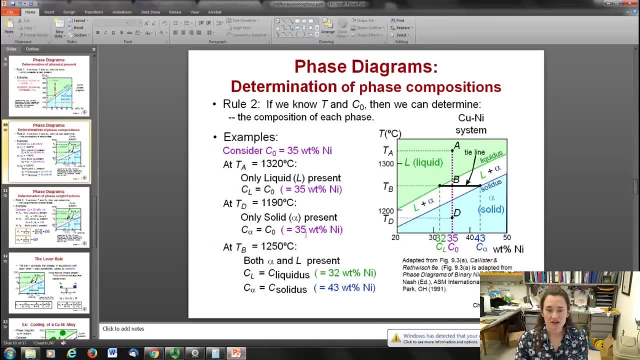 middle here and I have a liquid plus an alpha phase, So it's a mix of liquid and solid there. So I can easily read these off. That's not a problem. Rule number two: if I know the temperature and the percent composition, then I can determine the composition. 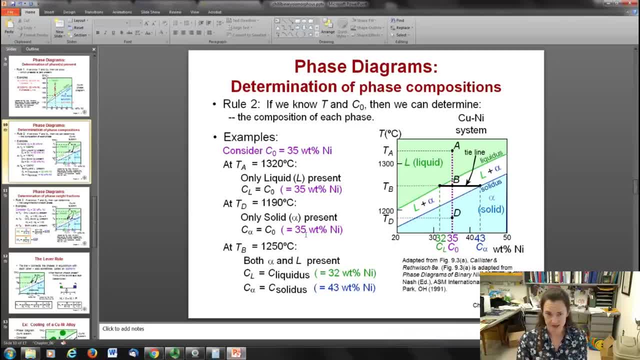 of each phase. okay, All right. now this is a little more complex. Let's do the easy ones first. Let's go to point A up here in the liquid region. okay, If I'm at point A, then I'm at 35 weight. 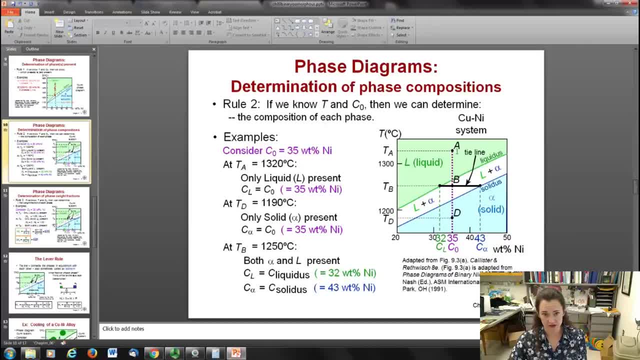 percent nickel. okay, So I have 35 weight percent nickel and I have only the liquid phase present at 1320 degrees C. So my liquid is my whole phase and it's the liquid that's present at 1320 degrees C. So my liquid is my whole phase. 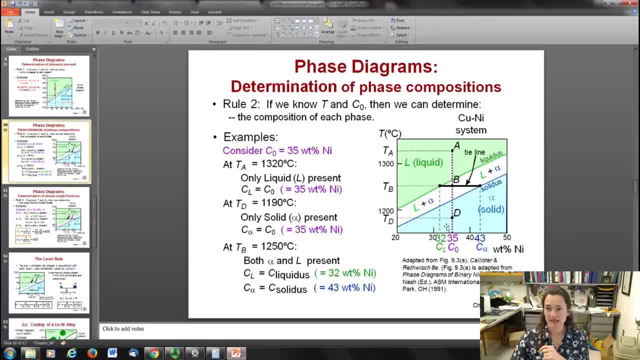 and it's the liquid that's present at 1320 degrees C. So my liquid is my whole phase, and it's 35 weight percent nickel. okay, Now let's go to another easy one. Let's say I'm still at 35 weight percent nickel, but now I'm at a temperature of 1190 degrees C. 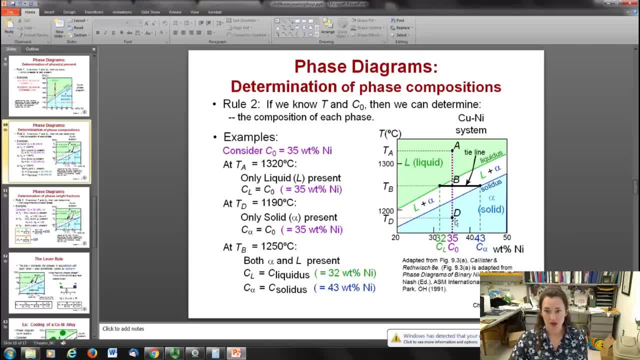 That puts me down here in the solid region. okay, So I've got only solid present, it's only alpha phase and it's 35 weight percent nickel. okay, So that's what it is. So that's pretty straightforward. But now let's go to this region B. okay, In the liquid. 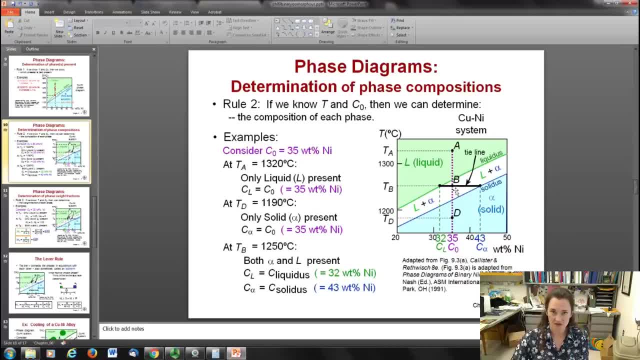 plus alpha phase G Right, I'm actually interested to understand if a liquid will reveal its region. So I know I have alpha phase and liquid phase. Now what I'm going to do is I'm going to construct what's called a tie line, And a tie line is a horizontal, straight, flat line on the 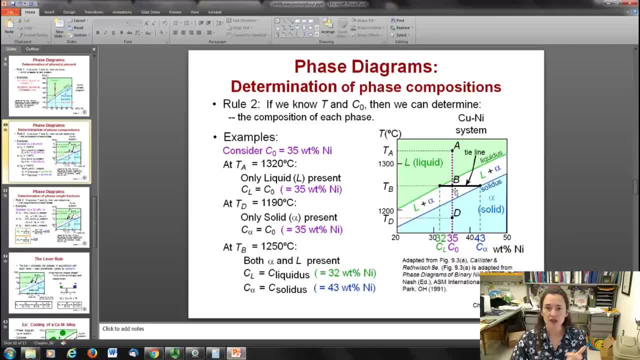 scrap. It's also sometimes called an isotherm And I'm going to look at the intersection of my tie line with my liquidus line here, which defines the boundary between the liquid and the liquid plus alpha phase, and my solidus line over here, which defines the boundary between my liquid plus. 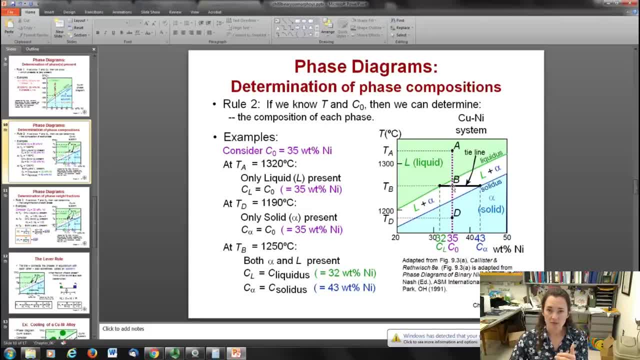 alpha phase and my alpha phase. Okay, Now I'm going to read off what the concentrations are at the intersection of the tie line with the liquidus line and the solidus line, And from that I can extract some information. So the concentration of my liquidus phase is, if I go. 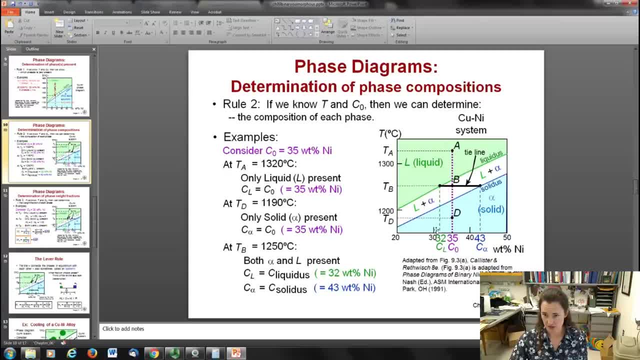 over and look at the intersection with my liquidus line and I drop down and see what the concentration percentage is at that intersection point. then I see it's about 32.. Okay, So that means that the concentration of my liquid phase in this liquid plus alpha region at 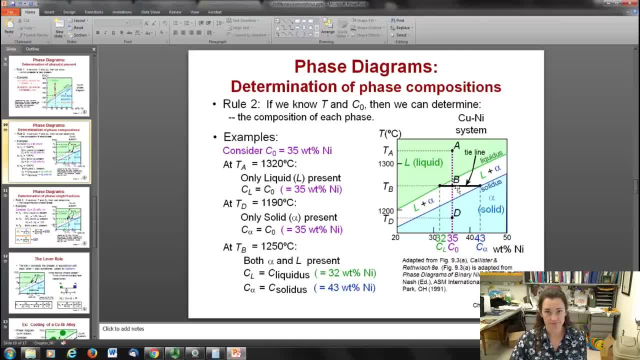 this very specific temperature is 32 weight percent nickel: Okay, Now if I go across and look at the intersection of my tie line with my solidus line, then I can see that it intersects at a concentration of 43 percent. Okay, What that means is that the alpha phase that's present there 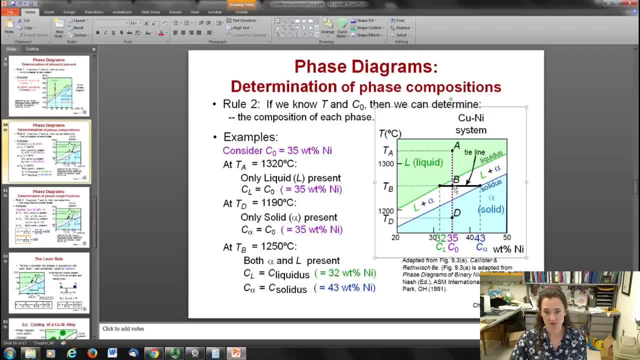 has a concentration of 43 weight percent nickel. Okay, Now, if you think about it, this kind of makes sense. All right, So we have a phase diagram that shows us that the melting point of copper is lower than the melting point of nickel. So if you're in this region, okay. 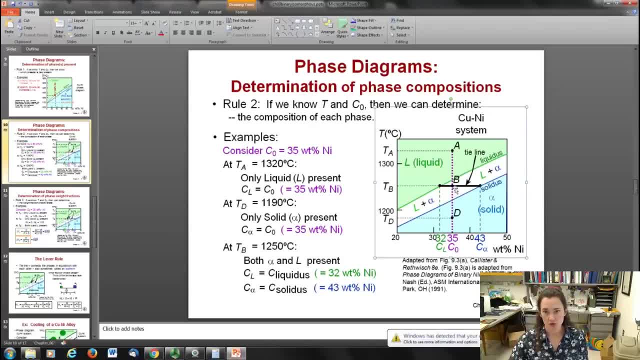 if you're in this middle region, then you know that you've probably had more copper melt than nickel. Okay, So that means that the weight percentage in your liquid phase is going to be lower. right for nickel, because it hasn't melted as much yet, And the weight 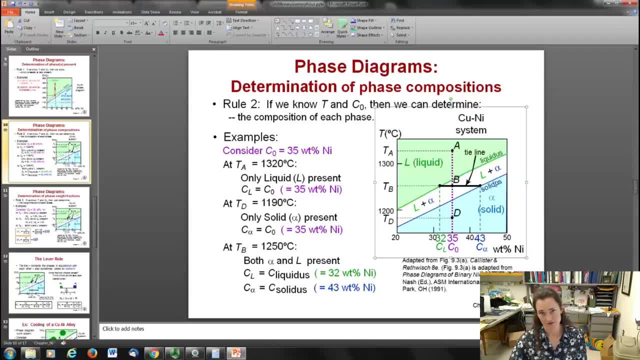 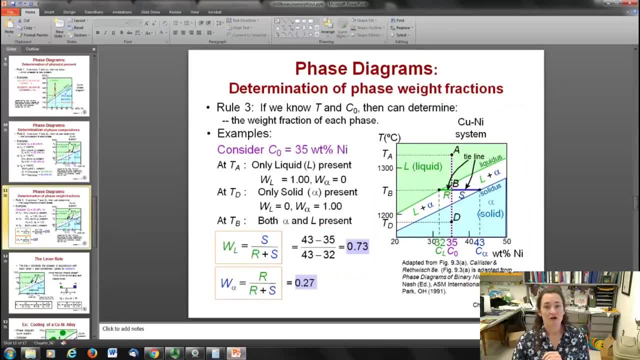 percentage for my solid phase is going to be higher for nickel because nickel has a higher melting point. Does that make sense? Hopefully it does. Now you can get even more information. Rule number three: If you know the temperature and the percent composition. 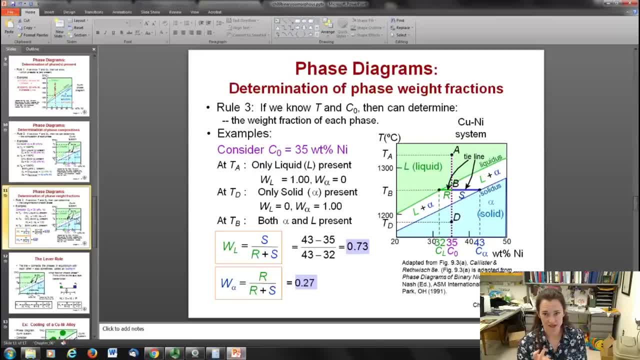 then you can determine the weight fraction of each phase. okay, So let's go back to our friend, the 35 weight percent nickel and look at its time line there at that temperature that we already looked at. So let's start with temperature A first, At temperature A. 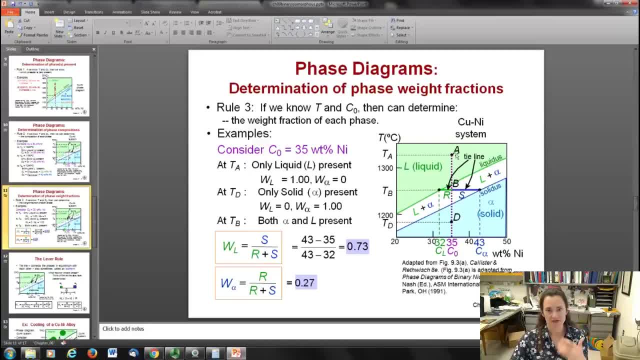 I've got 35 weight percent nickel and I've got 100 percent liquid. That's pretty straightforward. At temperature D down here I've got only solid phase, so it's 100 percent alpha phase and it's 35 weight percent nickel. But now, if I go back here to the middle at temperature, 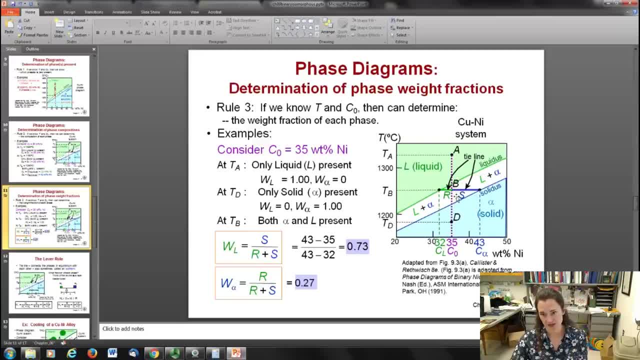 B, then I'll be at about where was I At, Luiza, Alright, So obviously I want to give. I know I've got alpha phase and my liquid phase present. I've got my tie line. My tie line intersects at 32 weight percent on one side and 43 weight percent on the other, But I'm sitting right here. 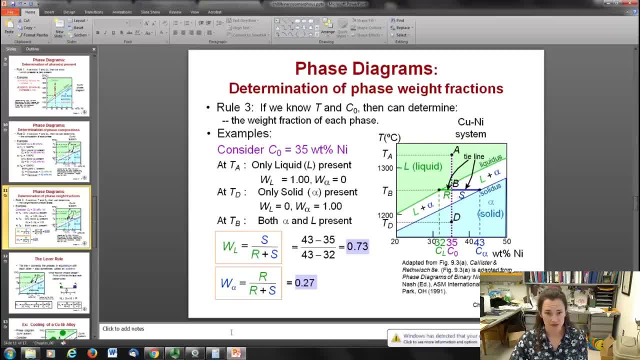 at 35 weight percent. So I know that I can figure out what weight percentage of liquid I have in that liquid plus alpha phase and what weight percentage of alpha phase I have in that liquid plus alpha phase. So I can tell you not just that I have alpha phase and liquid phase, but what. 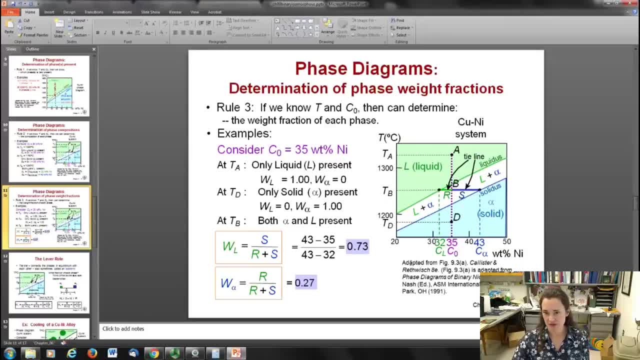 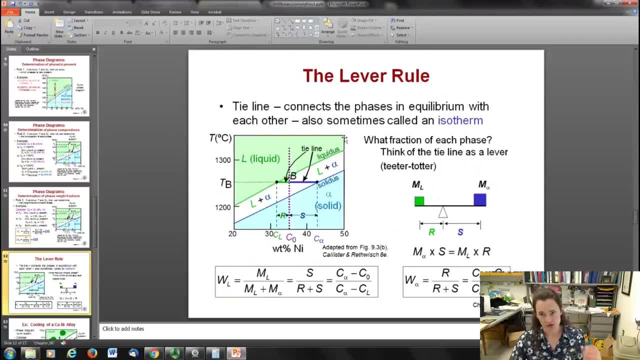 weight percentages. those two things are. I can do that by using my tie line and what's known as the lever rule shown here, So the tie line connecting the two, also called an isotherm. what you can do is you can look at the relative weights of the liquid versus the alpha phase based on the tie. 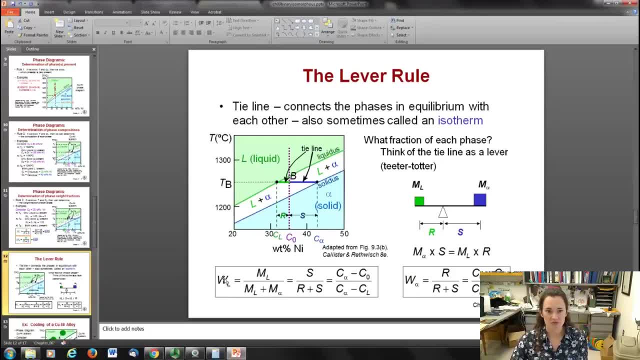 line. So if you want to calculate the weight percentage of the liquid in that liquid plus alpha phase, then you look at what concentration you're at. You're at 35% and then you compare the relative lengths of your tie line before it intersects the liquidus and solidus lines. 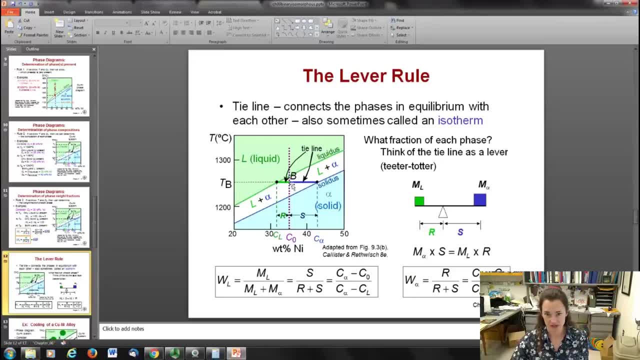 You can compare the relative lengths of that and get a weight percentage out of it. So let's look at our tie line. If we consider R to be the distance on our tie line from the intersection of the liquidus line to the concentration that we're at and we consider S to be the length of 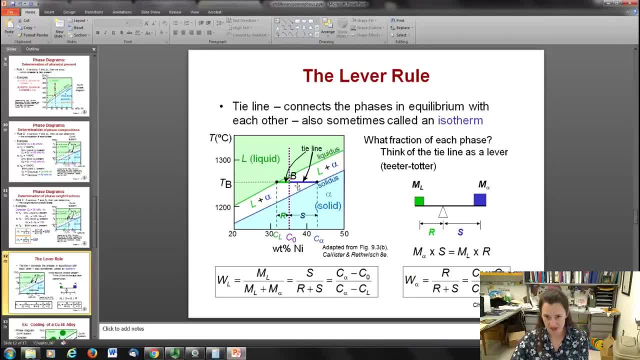 our tie line from the weight percentage that we're at 35% to the intersection with the solidus line. then I can find the weight of the liquid phase by the calculation S over R plus S. S I can find by looking at the concentration at the intersection with the solidus line, C-alpha. 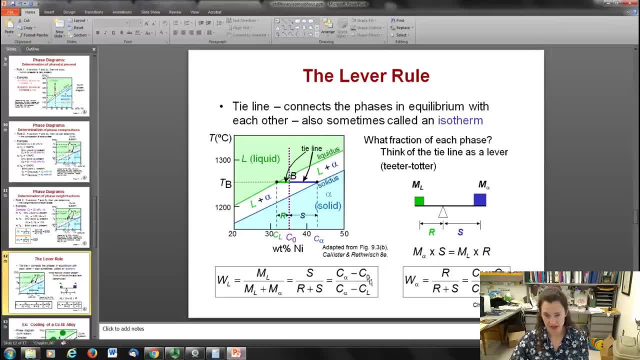 minus the concentration that I'm at, which is 35%, and then I divide that by the total length of my tie line from the liquidus to the solidus lines, which is the concentration at that alpha phase intersection minus the concentration at the liquidus line intersection. 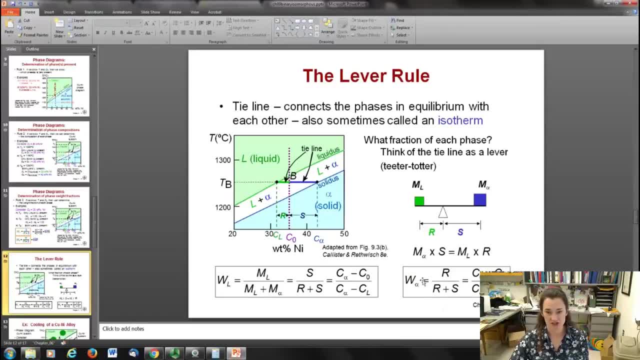 Okay, And then I can do the same thing if I want the concentration of my alpha phase. Instead of S over R plus S, I do R over R plus S. All right, Does that make sense? Okay, so I can figure that out. 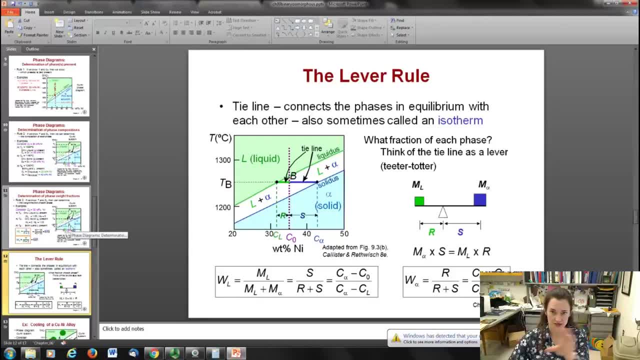 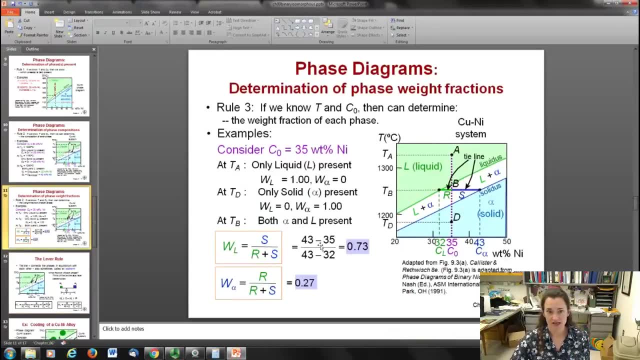 Now from this slide- it was all constructed here breaking it down- but if I run through the calculation for the weight of my liquidus phase, I get S, which is 43 minus 35, divided by R plus S, which is 43 minus 32, and I see that I've got 0.73, or 73% liquid. okay, at. 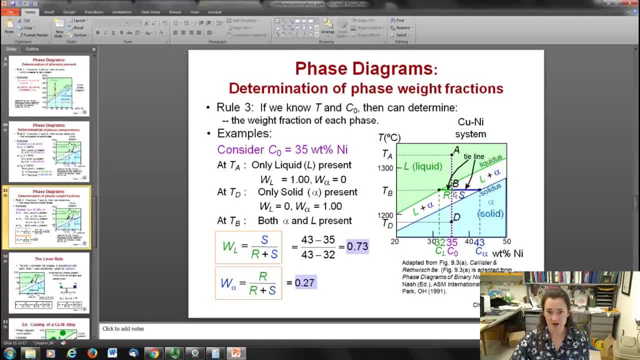 that point And that kind of makes sense that I'm going to have a higher percentage of liquid at that point, Because I'm really closer to the liquidus line than I am to the solidus line. Okay, So it makes sense that I have more liquid than solid. 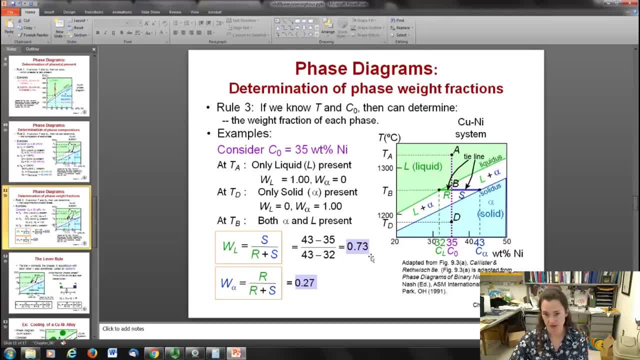 And of course, if I have 73% liquid, then I've got 27% solid. but if I wanted to verify that, I could just do R over R plus S, which would be, you know, 35 minus 32 over 43 minus. 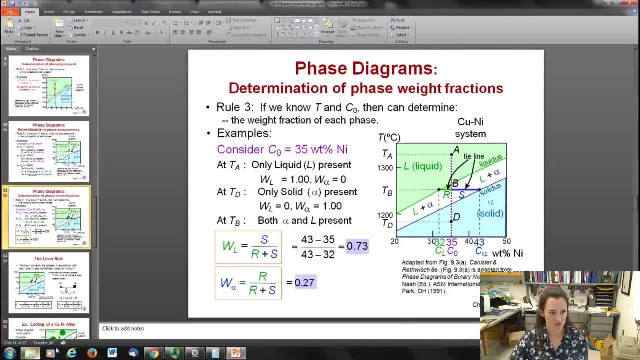 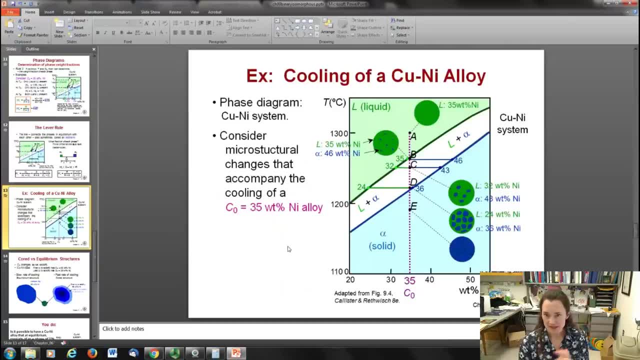 32, and I would get 0.27.. All right, I hope that's relatively clear. Okay, So what happens is: let's look at what happens in a vertical line. So we're holding constant at 35 weight percent nickel and we start out in the liquid phase. 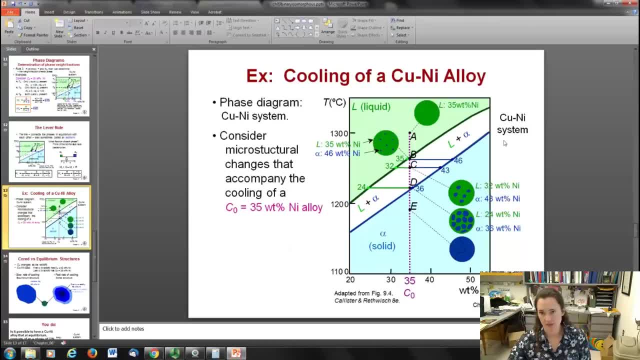 and then we slowly cool it down and watch what happens. Okay, So I'm up here, I'm very far away from the liquidus line and I'm at 35 weight percent nickel, And now I start to cool it down kind of slowly. 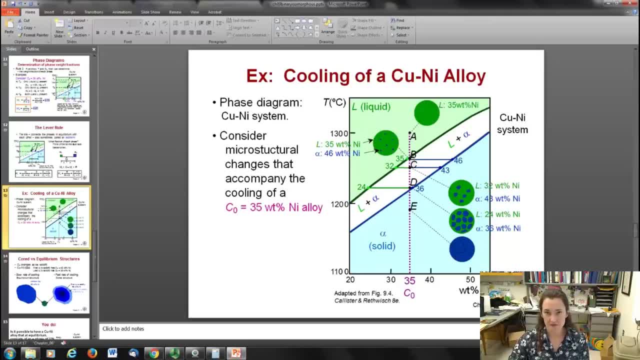 When I reach my liquidus line. okay, Then I get the formation, And I get the formation of some little solid phase particles, okay, That's indicated in this little cartoon over here. In this cartoon the liquid is shown in green and the solid alpha phase is shown in blue. 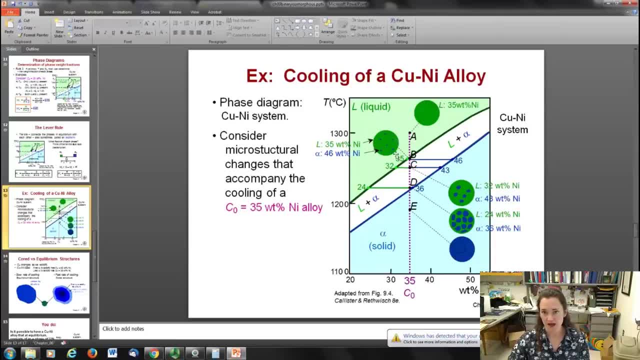 So at B I'm starting to see these little tiny alpha phase solid particles forming. Now, given where the thing is okay, if I construct a tie line here and look at the intersection on either side, I've got 35 weight percent nickel for my liquid phase. and then 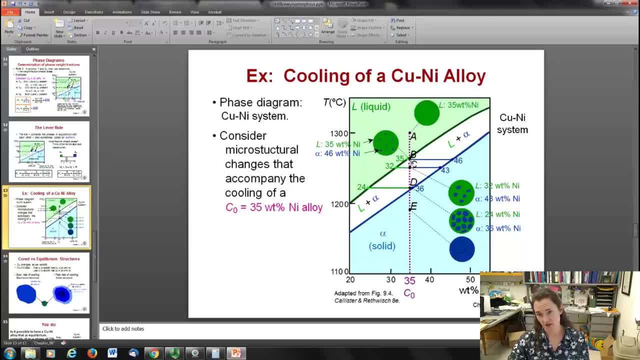 for my alpha phase. if I go across here and draw my tie line and construct to go to the other side, then I've got 46 weight percent of nickel. So because my nickel has a higher melting point, the nickel is going to preferentially. 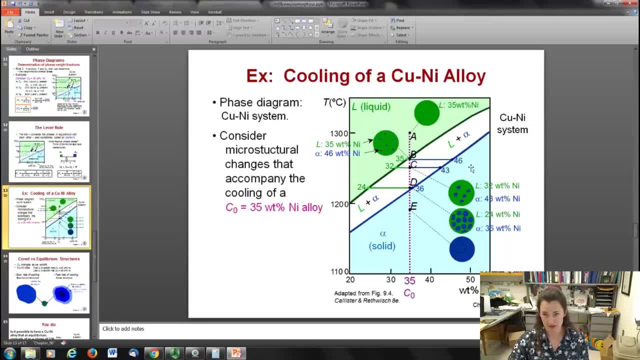 become a solid first. okay, It's going to preferentially become a solid first, And so these little particles are going to be very nickel rich compared to the bulk concentration of the liquid, which is 35 percent. Okay, So now let's say that I drop down a little further. 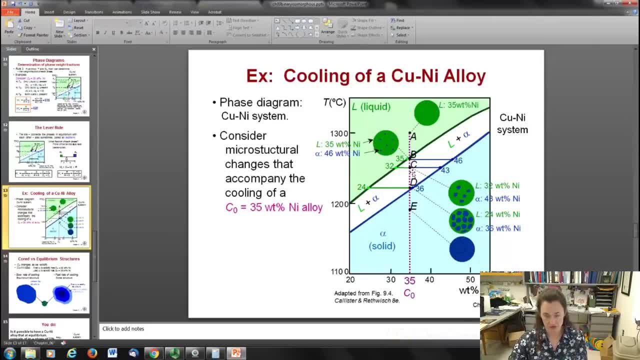 Well, if I look at what my tie line looks like here- okay, I've cooled down more. Now, if I construct my tie line, my liquid phase is 32 percent nickel and my solid phase is 43 percent nickel. And as I go further and further down, I see the weight percentage of the nickel drop until 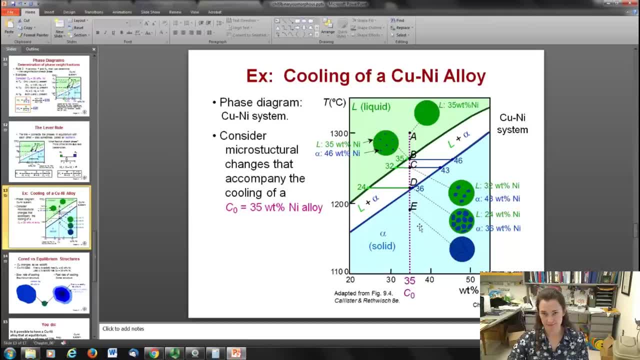 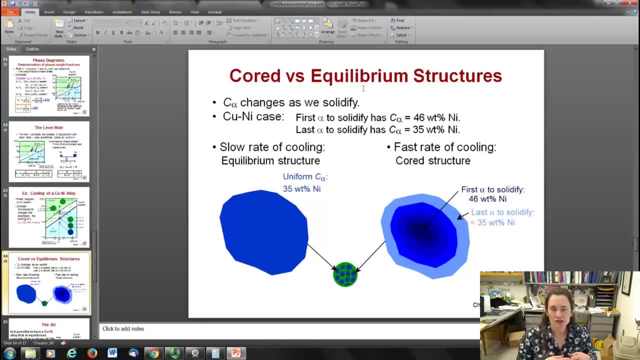 when I reach the solid region, it's 35 percent again. okay, All right. Now what does that mean? really Well, If you cool it down in an equilibrium kind of way, not much. Basically, what'll happen is, if you do it slowly enough, your copper and nickel diffuse and 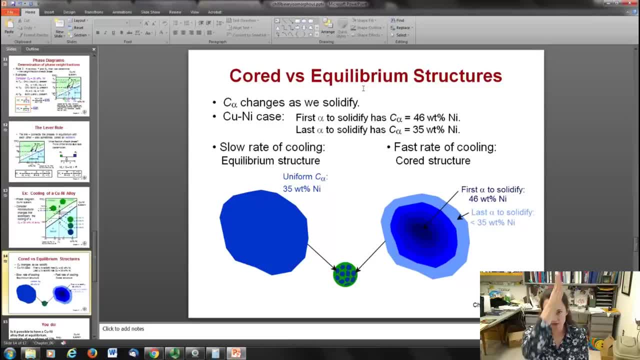 move around and you'll have a homogeneous mixture by the time you get down into the solid phase temperatures, and it'll be 35 weight percent nickel, no matter where you are Okay. So that's at a very slow rate of cooling, though, that you get those equilibrium structures. 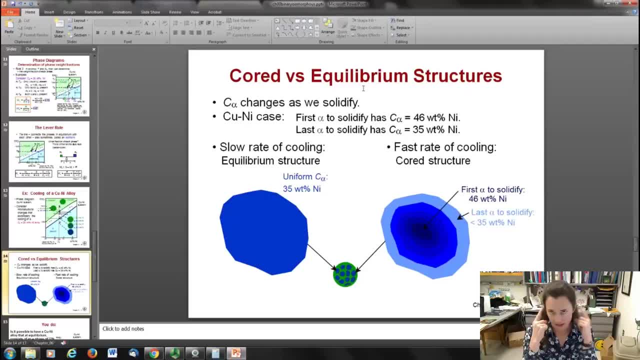 Any time you hear the word equilibrium In any sort of thermodynamics class, you should think: slow, painfully, painfully slow. That's what equilibrium really means. okay, Things have been given time to equilibrate. Now this is also rare, because in a real manufacturing facility or any kind of thing like that, people 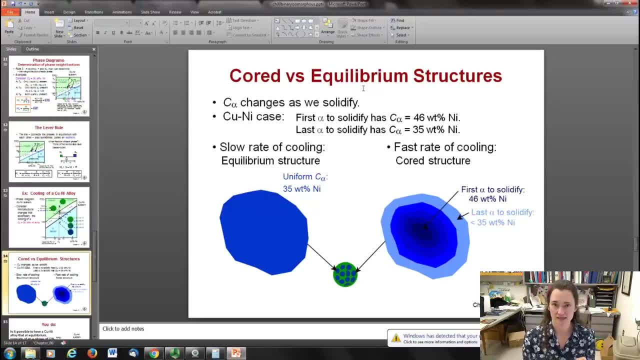 are not that patient. They want results, They've got money, They've got deadlines, And so things usually aren't at equilibrium-type conditions, okay, So what happens when you're not in an equilibrium position? Equilibrium condition is that the diffusion of the copper and nickel moving around it. 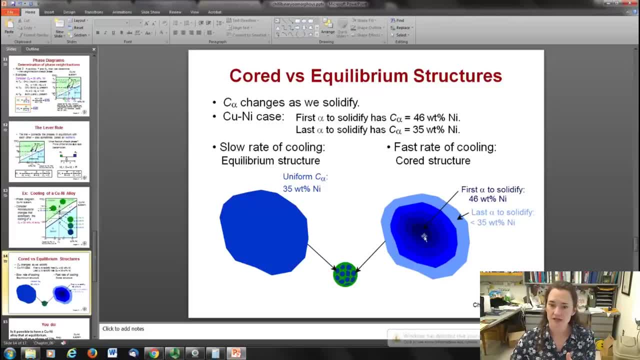 doesn't have time to happen, okay, And so when it starts to cool in the very core, when the nuclei first form, you've got a very nickel-rich phase, And then, as you move outward, then you're going to decrease the percentage of nickel. 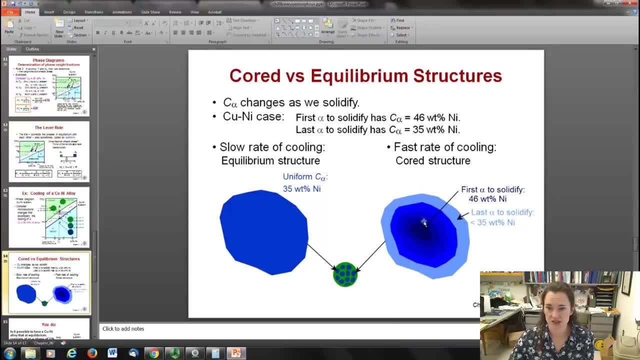 as you move outward. So in a lot of these regions you're gonna see a nickel-rich phase on the inside and then sort of a chord shell structure And that's where the percentage nickel drops off as you cool it down and as the solid. 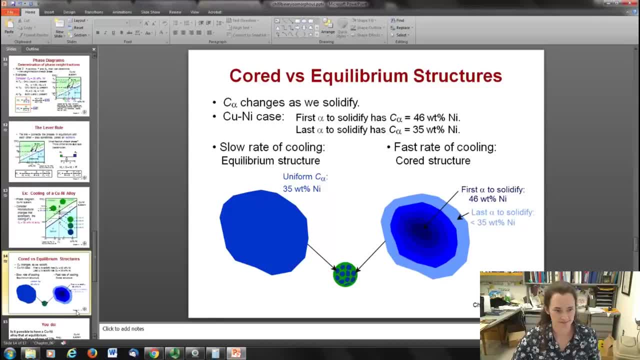 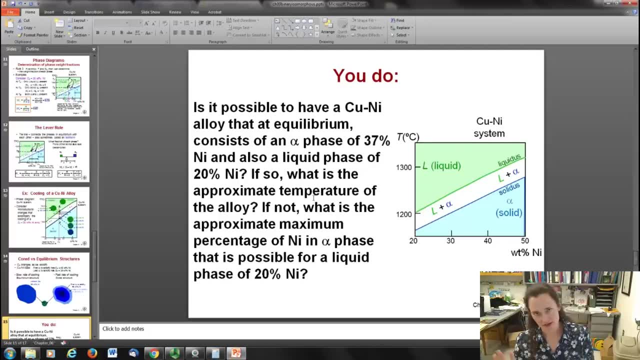 phase moves away from the nucleation site. okay, So what kinds of homework questions can possibly be asked about this? All right, here's an example problem: Is it possible to have a copper-nickel alloy that, at equilibrium, consists of an alpha? 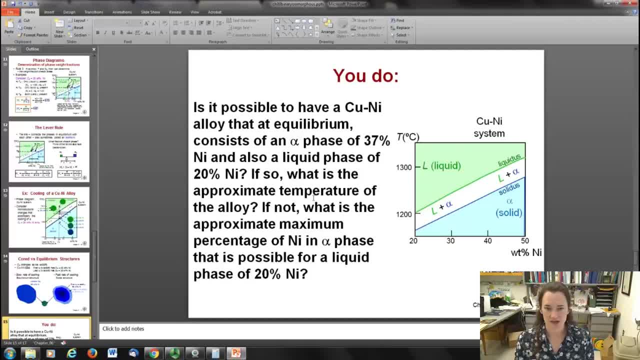 phase of 37% nickel and also a liquid phase of 20% nickel And if so, what temperature? What temperature is that alloy at? And if not, what's the maximum percentage of nickel in the alpha phase that it's possible for a liquid phase of 20% nickel? 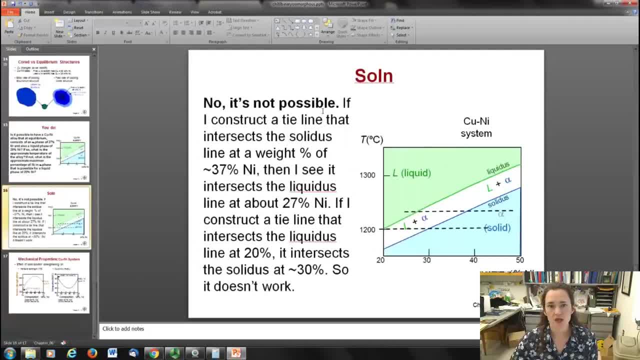 Okay, so here we go. It's not possible. all right, I've shown you why. here, I've got the diagram back up and I've constructed a couple of tie lines for you. So the first is I constructed a tie line, a horizontal line that intersected the solidest. 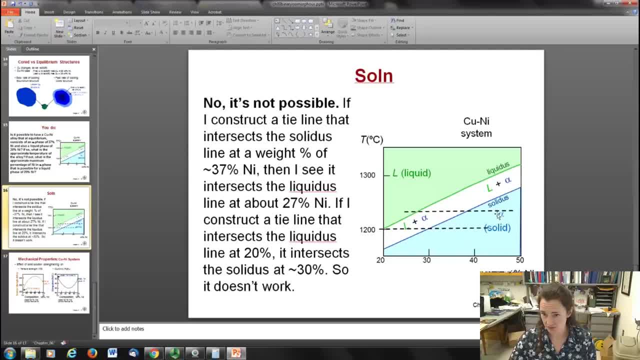 line at a weight percent of 37% nickel. So that's this top guy right here. It's intersecting at about 37% nickel right there and you can see that. So that would mean that the alpha phase would be 37% nickel. 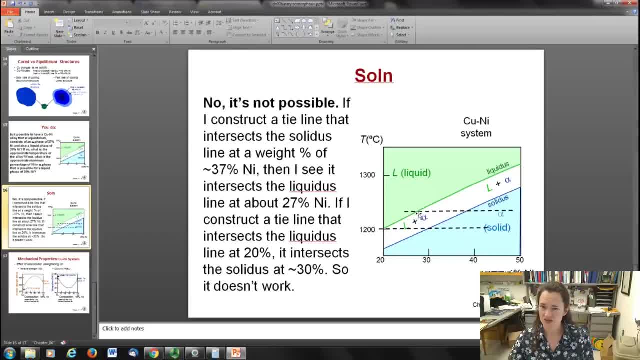 But if you go across to where it intersects the liquidus line, then you can see that the best it can do is, say about 27% nickel in the liquidus phase, So you're not going to get it. okay Now if instead you construct a tie line that intersects the liquidus line at 20%, that's. 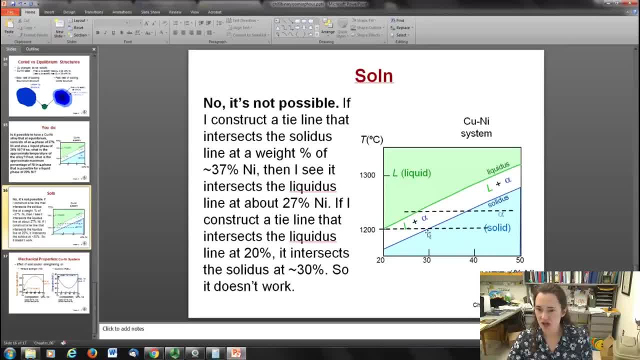 about right there, okay. Then it's going to intersect your solidus line at about 30%, okay. So the highest concentration of nickel that you'll get in your alpha phase is about 30%. So it's not possible, and instead the highest percentages that you'll get in the alpha phase. 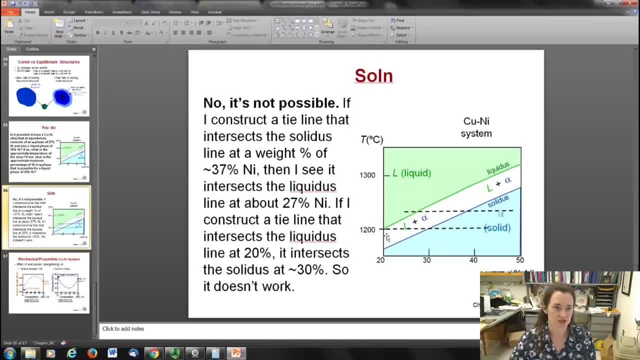 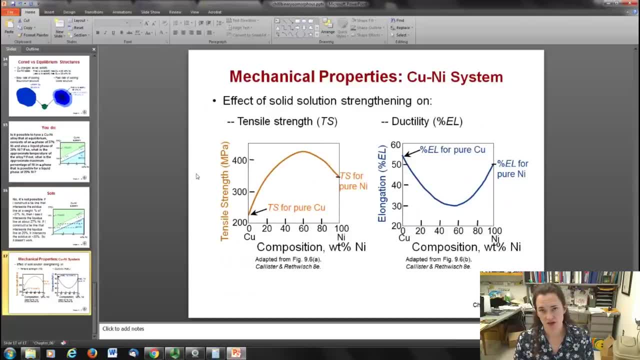 is about 30% for the 20% liquidus concentration. Okay, now, as you change the percentage of weight percent of nickel in this copper nickel system, you're going to see that you're going to get about 30% nickel And that's who you'll be okay. 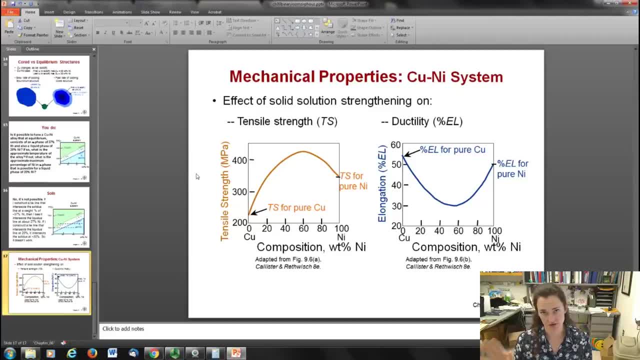 In some industry for a lot of this co توl factor. it can be wrong. okay, It's not something to worry about. The glaube in this theory. you know, put multiple times 20% nickel and it suns it in the total. 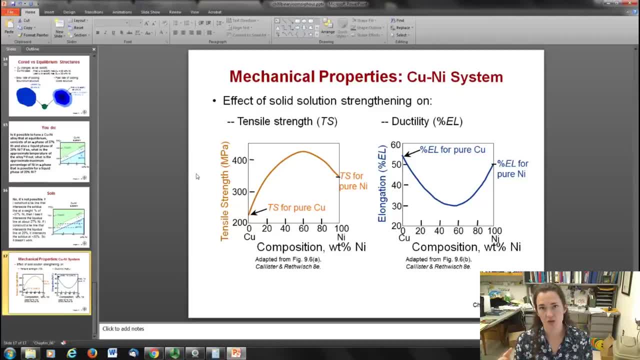 Elliott's 2- Jobs and still we'll, you know, just be aware of that. Okay, So we're going to let that cool down. So the idea, like you know, after 10% significant weight percent in this atom, then it's going. 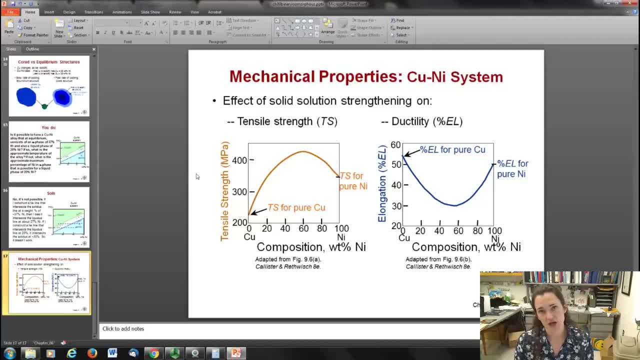 to affect various things. It's going to affect the tensile strength most dramatically and also the activity act as barriers to the motion of slip and dislocations. okay, so this dislocation can't move through. once it hits that dopant atom, it acts as a